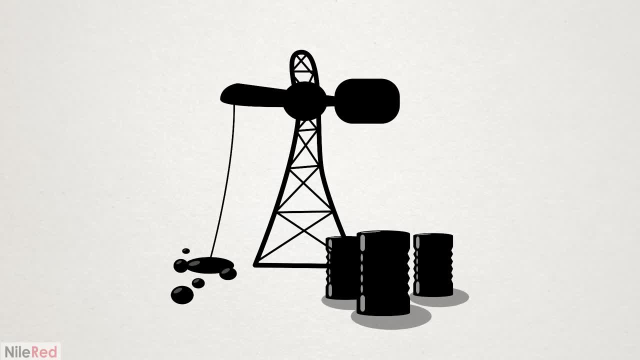 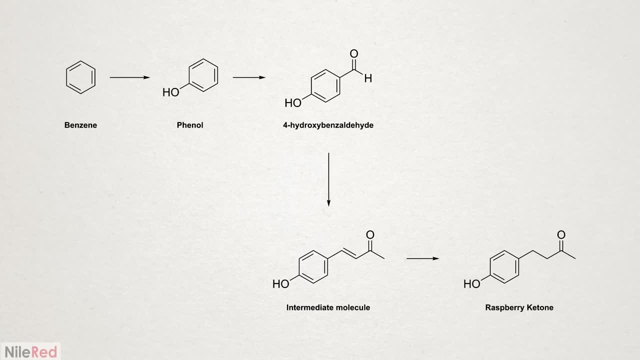 But with other flavors, fragrances and pharmaceuticals. the building process usually starts with some sort of cheap petroleum product. For any given molecule, there are many ways that it can be built, but for raspberry ketone, this seems to be the common pathway. 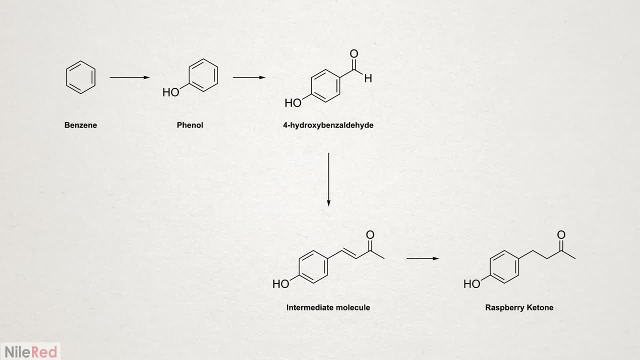 It starts with benzene, which is derived from crude oil, and with every step, the raspberry ketone molecule is slowly put together. This is a really long and labor-intensive process, though, and when producing it industrially, nobody's going to be starting with benzene. Like with most other syntheses, they'll start with the cheapest mass-produced precursor that's closest to the final molecule. In this case, it's often 4-hydroxybenzaldehyde. so that's what I'm going to be starting with. 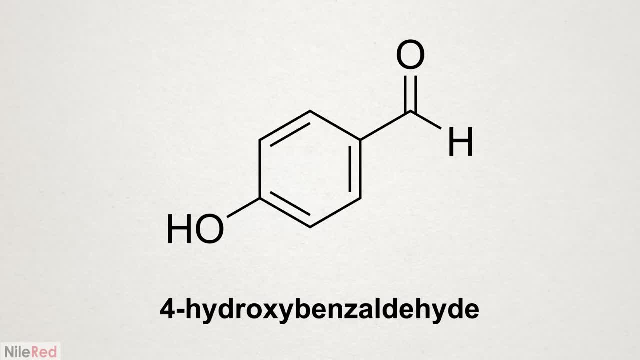 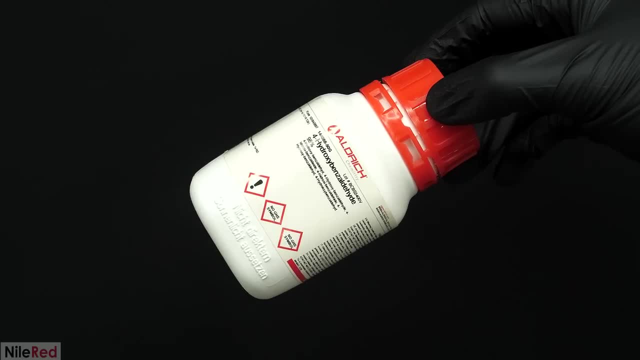 As usual, I tried my best to find an easy online source for this chemical, but unfortunately I wasn't able to find a single place. So I didn't really have a choice and I ended up having to order it from Sigma. So I didn't really have a choice and I ended up having to order it from Sigma. 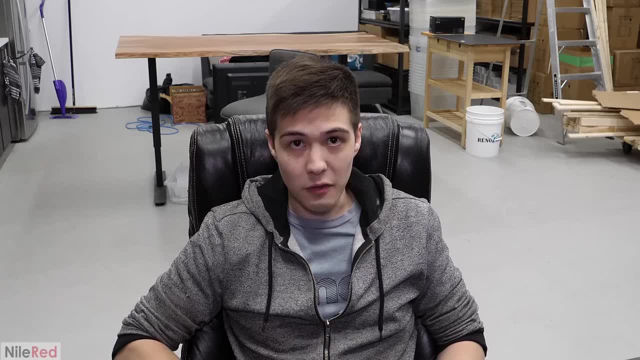 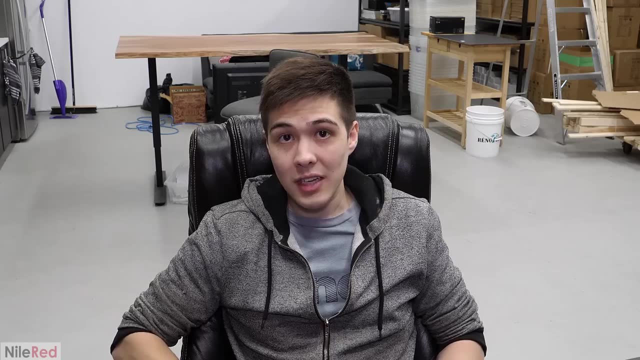 though I did just want to say that making the raspberry ketone myself was definitely not the most efficient way to make it. The entire point of this project was to just explore the chemistry and the science behind its production, and I thought that making it myself could just be. 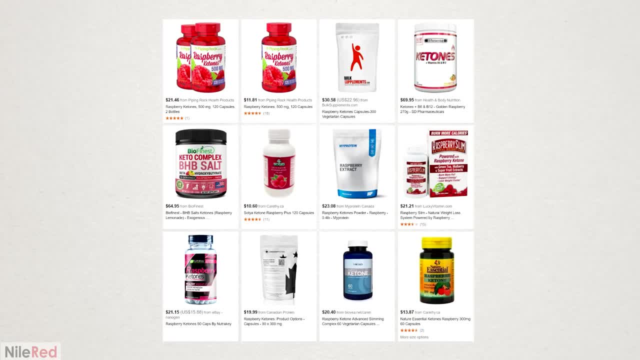 something fun to do. Unlike the 4-hydroxybenzaldehyde, the raspberry ketone is actually quite easy to buy online. There are a lot of places that sell it for cheap, but it's not meant to be used in food or perfumes or anything else like that. It's instead sold as a weight loss. 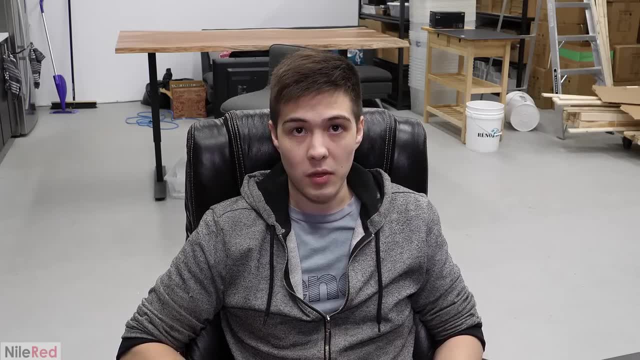 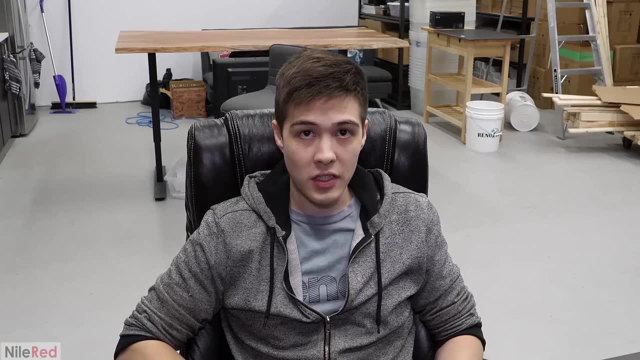 supplement, but as far as I know, as with many other weight loss supplements, there's no evidence to support that it works. However, it was convenient for me to have an easy and pure source of the ketone, and you'll see later on in the video how I take advantage of this. 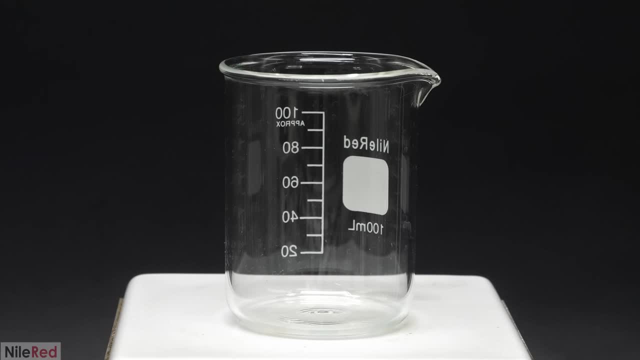 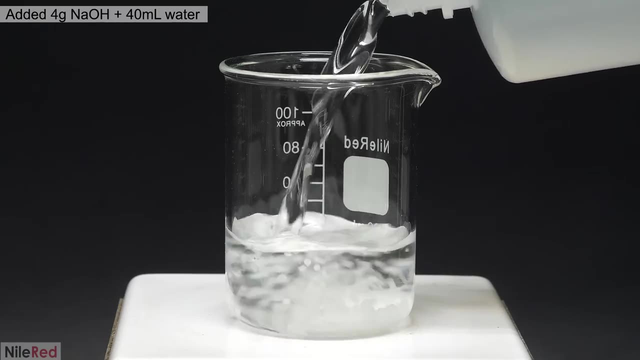 But anyway, with that being said, we can finally get started. The first step was to make a dilute solution of sodium hydroxide, so I added about 4 grams of it to a beaker, followed by 40 mils of. 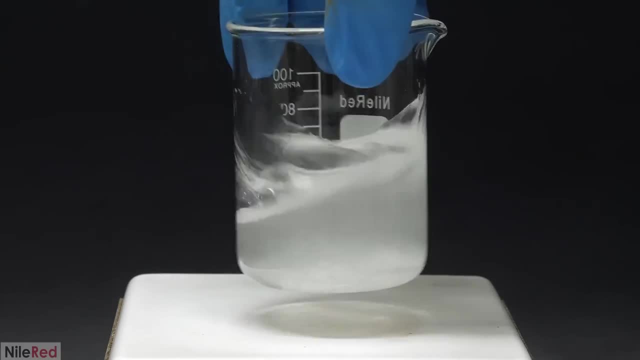 water. I swirled it around a bit over the course of a couple minutes, and then I added about 4 grams of it to a beaker, followed by 40 mils of water. Eventually, it all dissolved. I didn't need this solution right at the moment, though. 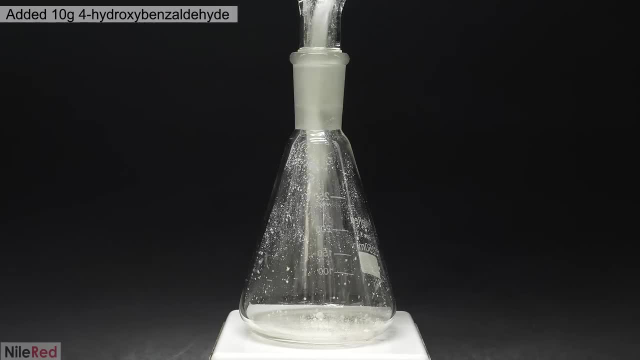 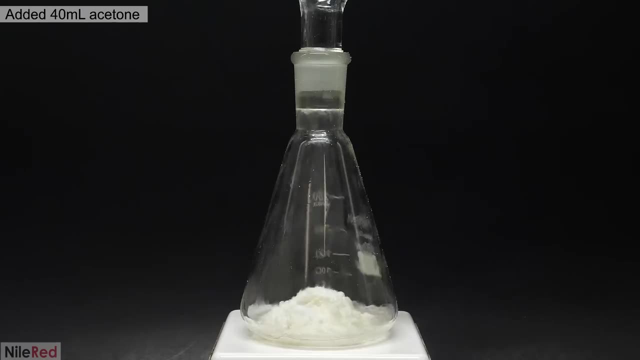 so it was temporarily placed on the side. I then got a flask and I dumped in 10 grams of the 4-hydroxybenzaldehyde. On top of this I dropped in a stir bar and I also added 40. 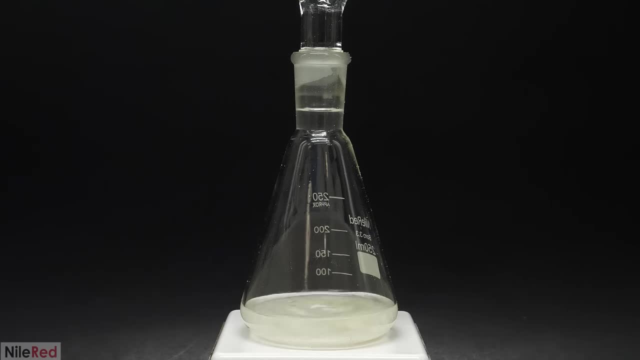 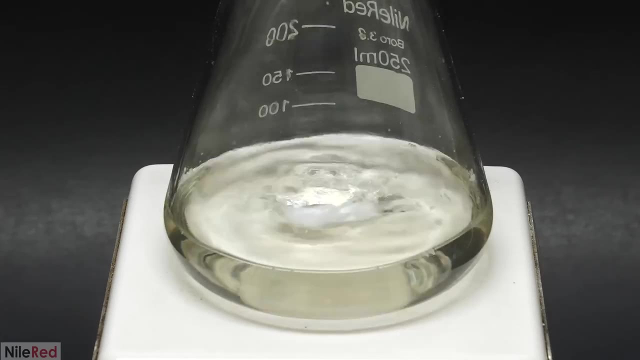 milliliters of acetone. It quickly dissolved a lot of the 4-hydroxybenzaldehyde, but to get the rest of it I had to turn on the stirring In. less than a minute later it had all disappeared. 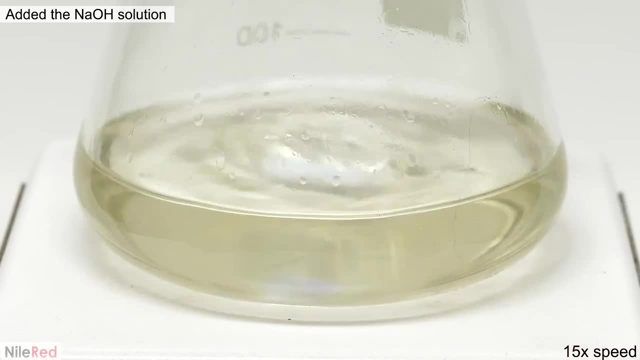 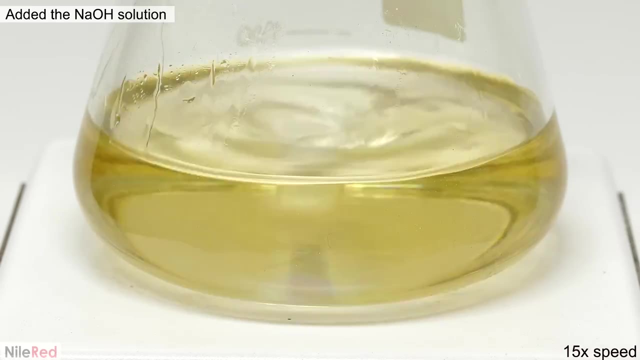 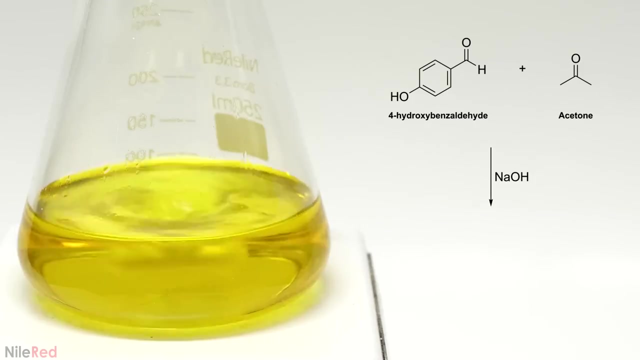 and I was left with this crystal clear solution. Now the next step was, with strong stirring, to slowly add the sodium hydroxide solution that I had just made before. This caused its color to slowly change and by the time that it was all added, it had turned yellow. What's going on here is a reaction between the acetone. 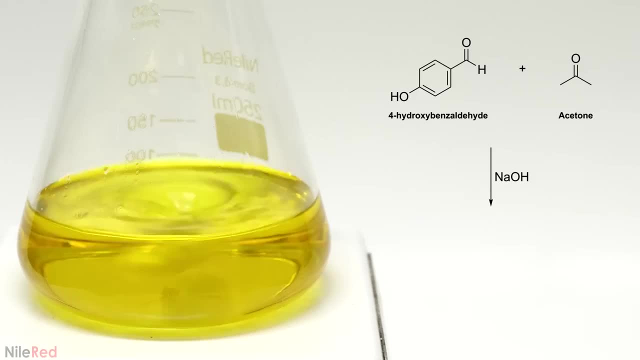 and the 4-hydroxybenzaldehyde, and it's catalyzed by the sodium hydroxide. This reaction is generally known as an aldol condensation, and a new carbon-carbon bond is forming between the two molecules. The result is this intermediate molecule. 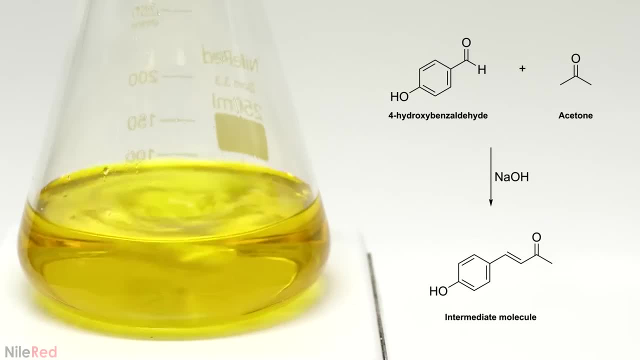 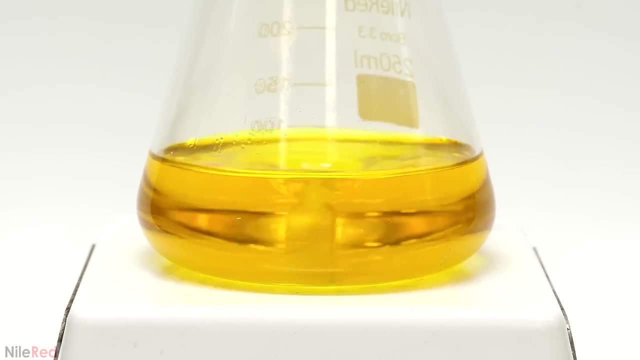 which is actually very close to the final raspberry ketone. However, it still has this double bond which I'll have to get rid of with another reaction. This intermediate has a slight yellow color and I think it's why the color of the solution changes. This reaction's. 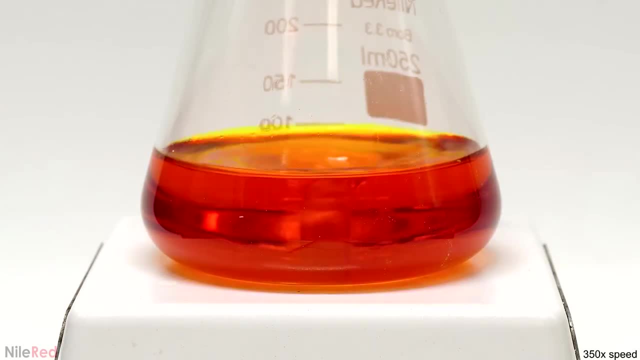 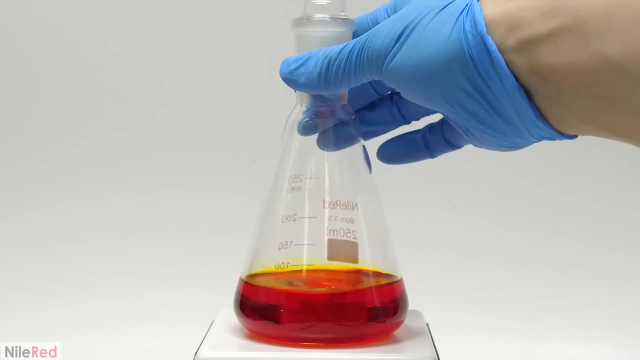 a bit messy, though, and it forms side products and tar, which I think cause it to slowly turn red. At this point I sealed it with a stopper, took it off the stir plate and I let it sit somewhere dark for about 24 hours. 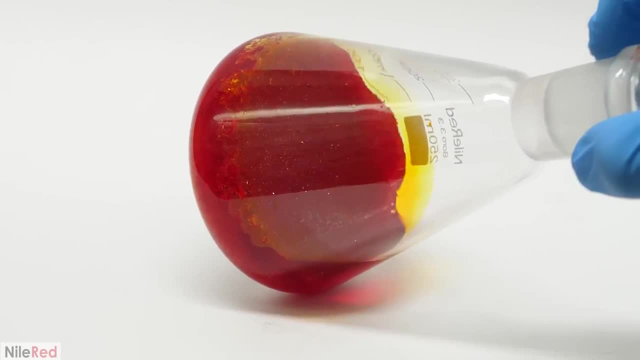 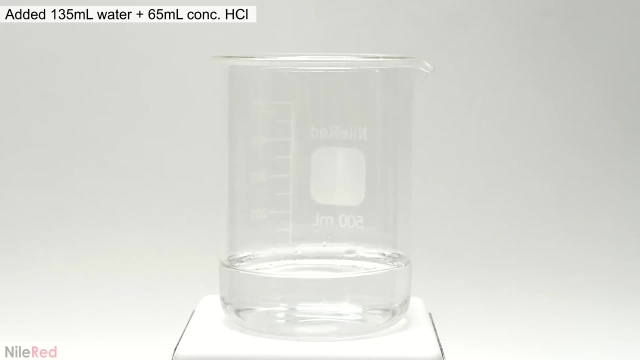 During this time the reaction slowly went to completion and when I came back to it it had almost completely solidified. Now into a beaker. I added about 100 ml of water, followed by 65 ml of concentrated hydrochloric acid. This was then topped off to about 200 ml. 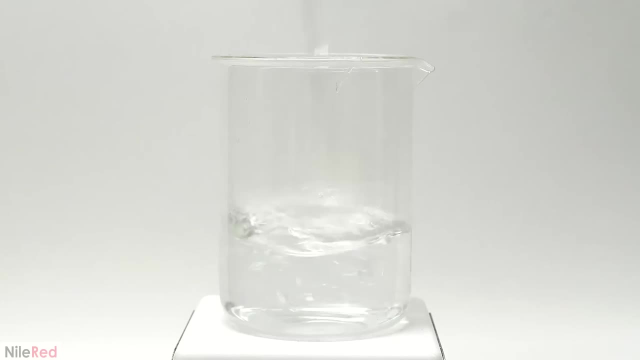 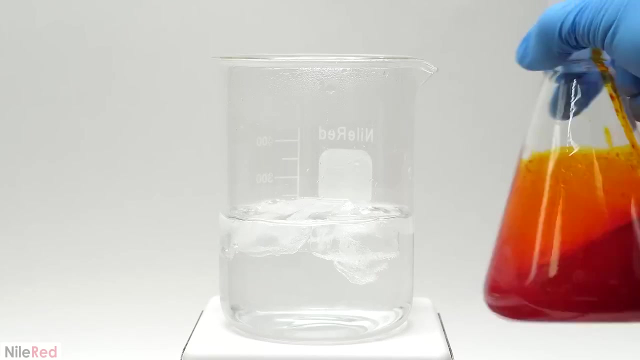 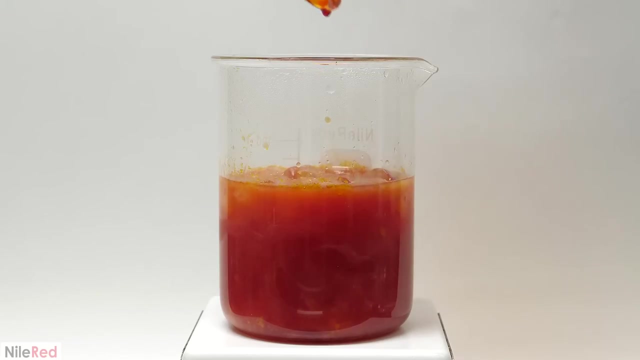 and it gave me roughly a 10% solution. This was all mixed together as thoroughly as possible and I also added some ice. Then I shook the reaction mixture to break up all the solid stuff and I poured it into the acid. The major reason for this step was to help purify out the raspberry ketone. 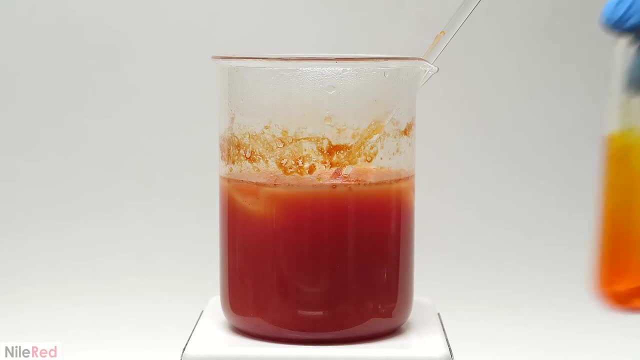 I also washed the flask a couple times with water just to get out as much as possible. This reaction isn't very clean and the base causes some of the acetone and our product to polymerize. Our desired product should have an off-white or slightly yellow color. 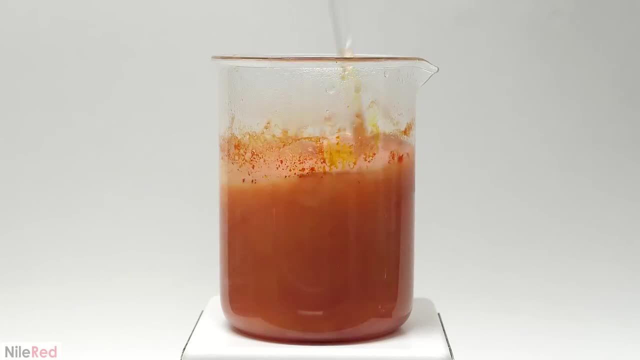 and I think that all this red stuff is just polymerized junk. By adding it to the acid, all the sodium hydroxide is being neutralized and it stops the polymerization process. This is a very important step to help purify out the raspberry ketone. 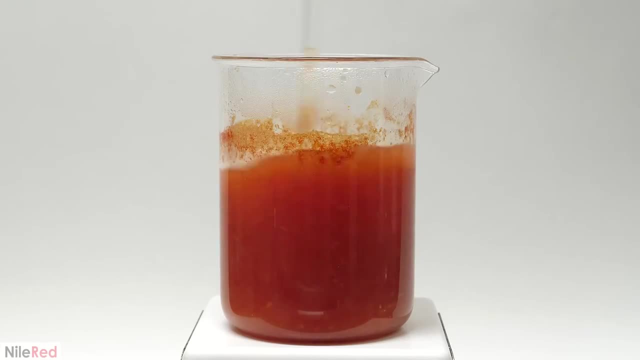 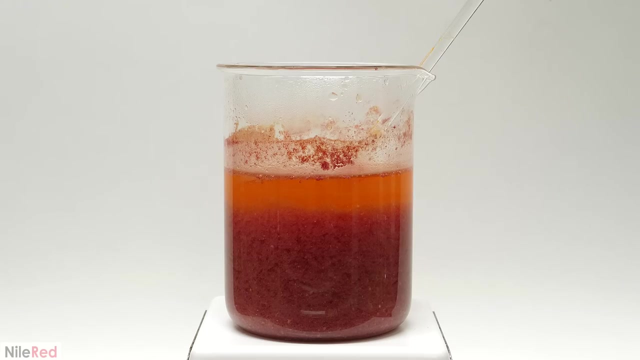 Also, the water dissolves the leftover acetone, which helps separate the product from the tar. This process didn't happen instantly, though, and the product just slowly crystallized out over the course of about 10 minutes. When it looked like it was done, it was time to get rid of all the water, and I did this. 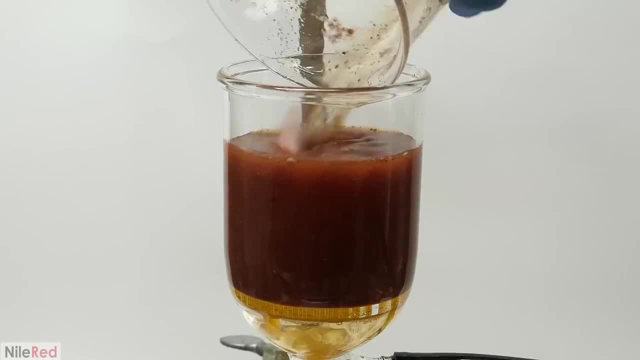 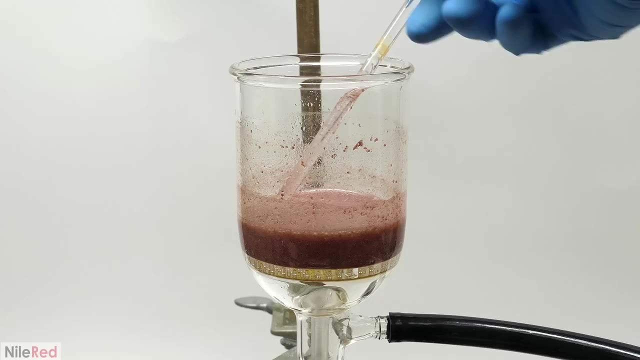 by vacuum filtration. So I turned on my vacuum pump and I started adding the mixture. When everything had been pulled through, I washed the beaker and the powder with some more water. Then I turned on my pump again and I let it run for a couple minutes. I was eventually. 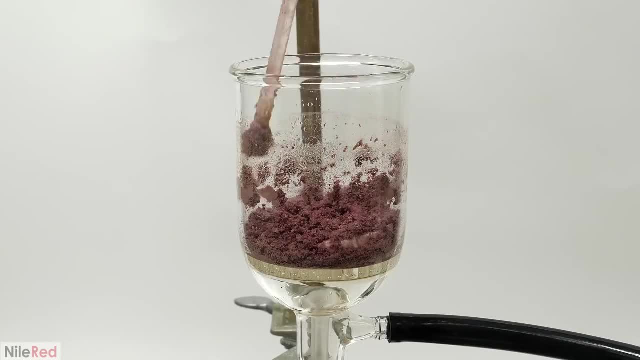 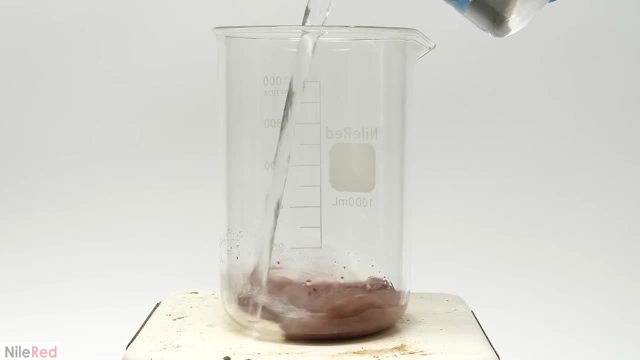 left with a reddish brown semi-dry powder, but it was still really impure. To clean it up, I just had to recrystallize it. so I poured it all into a beaker, Then I added a somewhat. 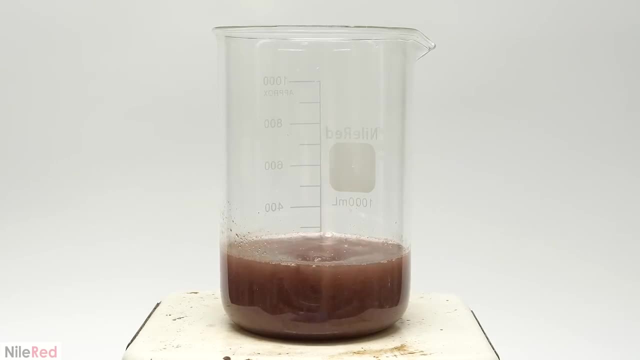 arbitrary amount of water and I turned on the stirring and heating. As it warmed up and got closer to the boiling point, more and more solid dissolved and it took on this green color Also. at some point all the solid had melted and it became a little bit. more solid. This is because the water was so hot and the liquid was not coming out. So I turned on my pump again and I let it run for a couple minutes and it became a little bit more solid and it took on this green color Also at some point. all the 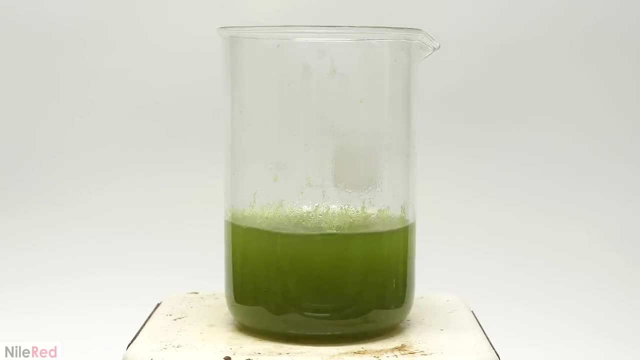 solid melted and it became an oily liquid. Most of it eventually disappeared, but to get the rest I had to start adding more water. I ended up adding quite a bit and at this point it looked pretty good, but there was still a small amount left. I really wanted. 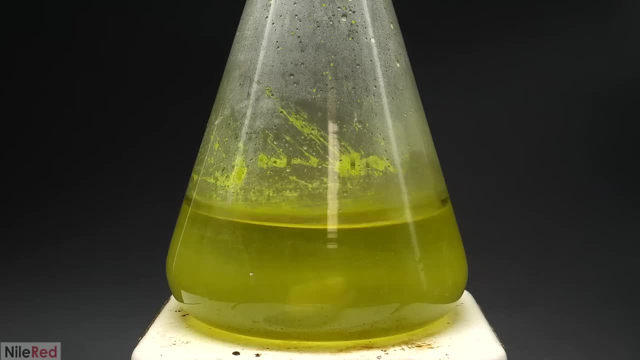 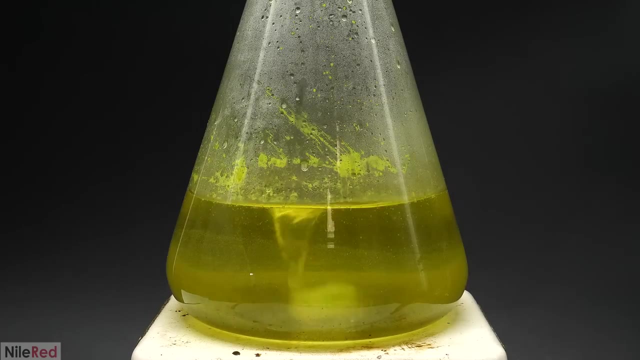 it to be nice and clear, but this would require adding more water and I worried it wouldn't fit in the beaker, So I just quickly transferred it to a larger flask and then continued adding more. It did end up clearing up completely, but it also didn't take that much more water. 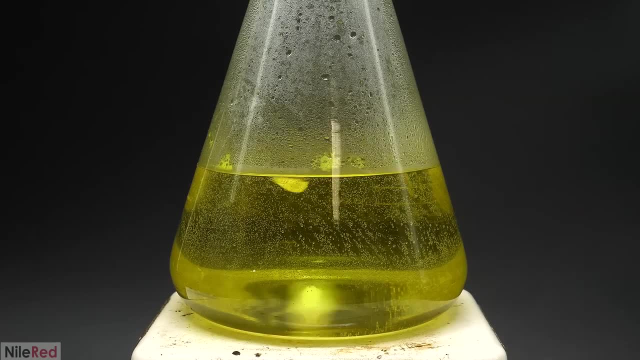 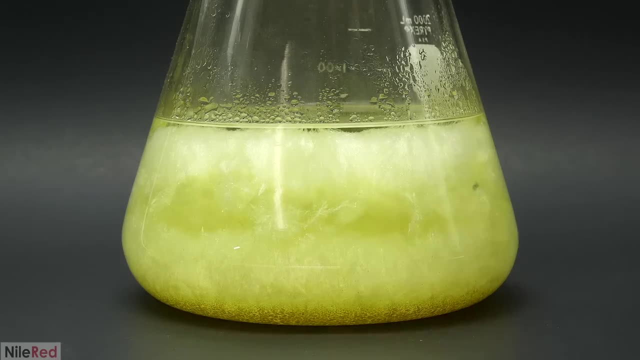 so probably everything would have fit in the beaker. but oh well, I then took it off the hotplate, pulled out my stir bar and waited for it to cool down. When I came back the next day I had a lot of nice whitish yellow crystals, but there was also a lot 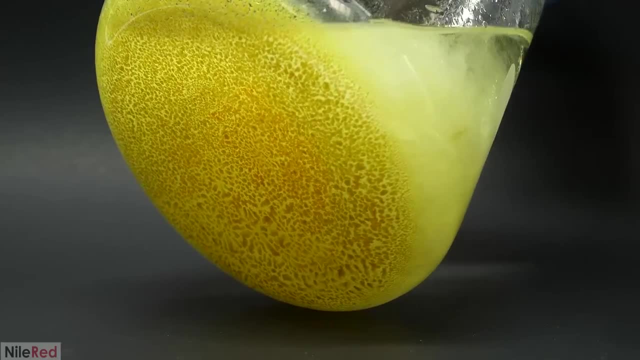 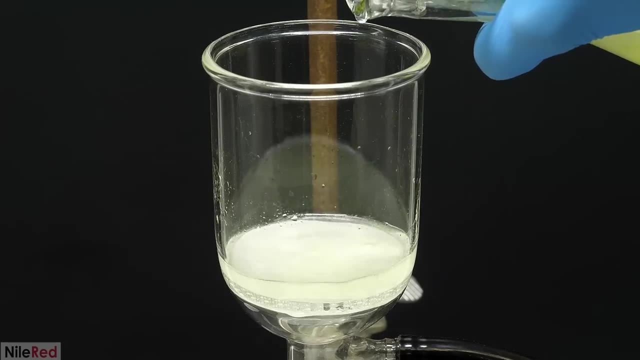 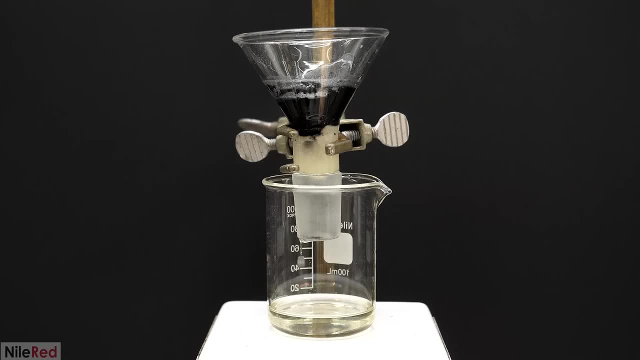 I was able to filter it off, and I was able to filter it off and I was able to filter fresh ethyl acetate. I've never had an issue with it. but one thing to keep in mind is that palladium on carbon is pyrophoric, meaning it can spontaneously ignite in air. This can sometimes 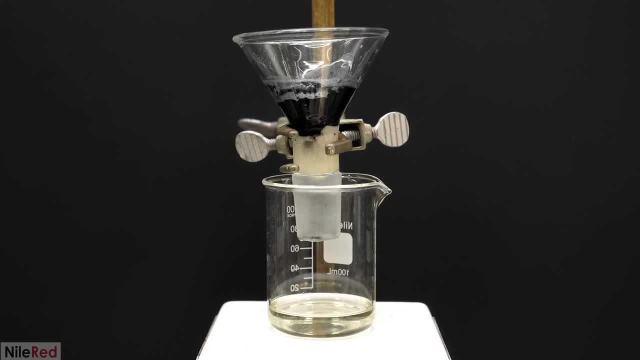 be even worse after the hydrogenation, because some hydrogen gets stuck to the carbon And what this all means is that it just has to be handled with care because it does pose a slight fire hazard. But anyway, with that all done, now I took away the funnel and I was left with this slightly. 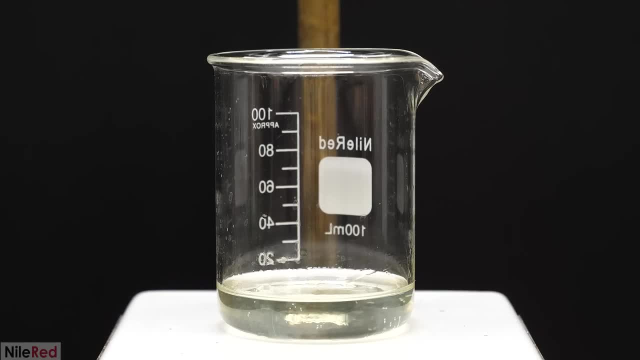 yellow solution. This contained all of the raspberry ketone that I made, and to isolate it I just had to get rid of the ethyl acetate. This was done pretty easily by just turning on the hot plate to a low heat and setting up a fan off to the side. Up until now, the smell was mostly overpowered. 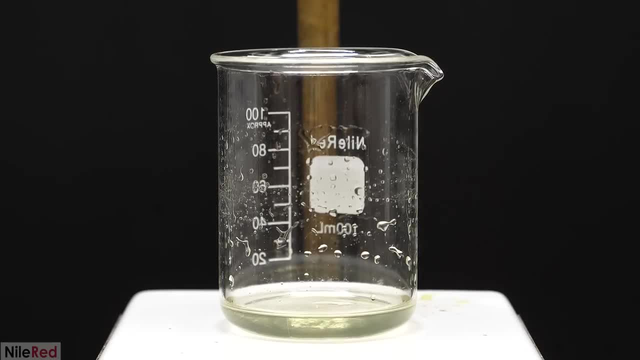 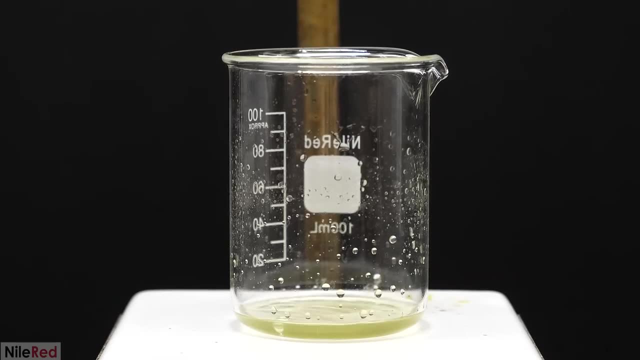 by the ethyl acetate, but as it was evaporated off and things got more concentrated, I started to smell raspberry. It was a very faint fruity and sweet smell and it was a lot like blue raspberry candy. It all disappeared in a few years, but a few months later they were gone As the time passed. 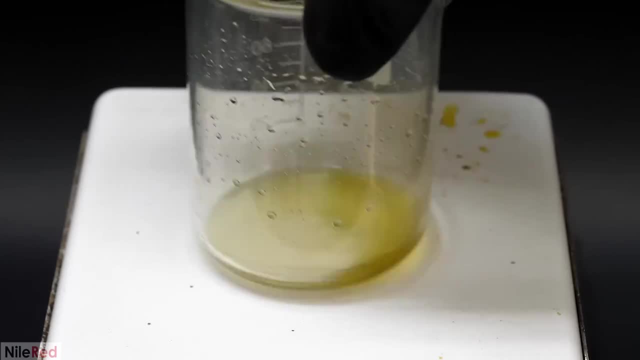 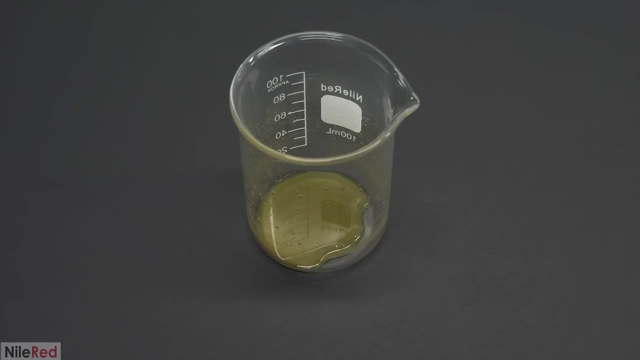 they were all gone and I showed up in this completely different state. I was also very. This appeared over the course of about 20 minutes and eventually, when I stopped smelling ethyl acetate, I took it off the hot plate. I was left with this oily stuff which I thought would crystallize as it cooled, but it just 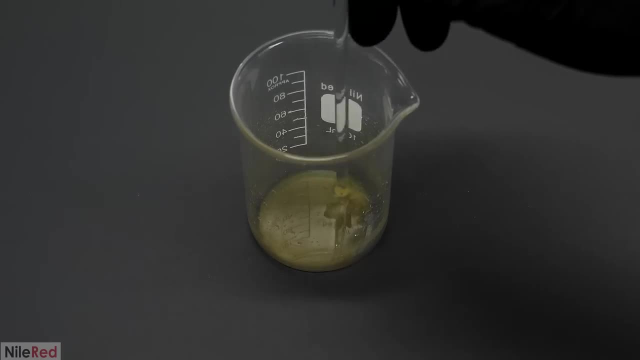 stayed as an oil. So to get it started, I got a glass rod and I scraped the bottom of the beaker. It initially didn't look like much was happening, but slowly I started seeing crystals forming. Then, over the next 30 seconds or so, the whole thing solidified. 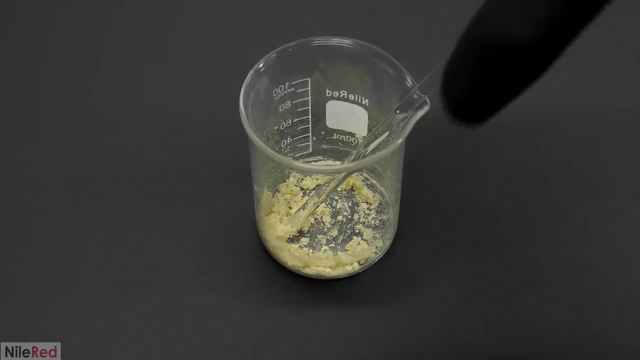 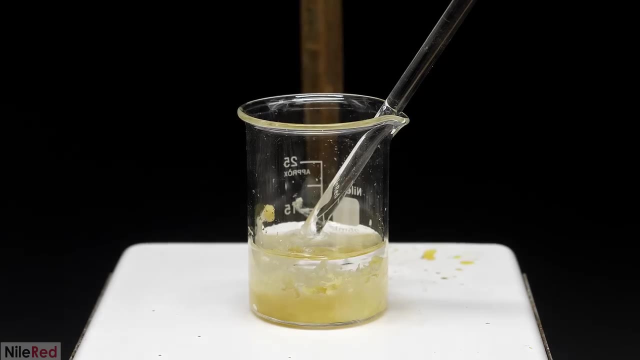 When using this rod, I was able to crush up most of it into this off-white yellowish powder. Pure raspberry ketone is white, though, so there are clearly still some impurities left over. However, from other runs, I found that it was really annoying to recrystallize, so I 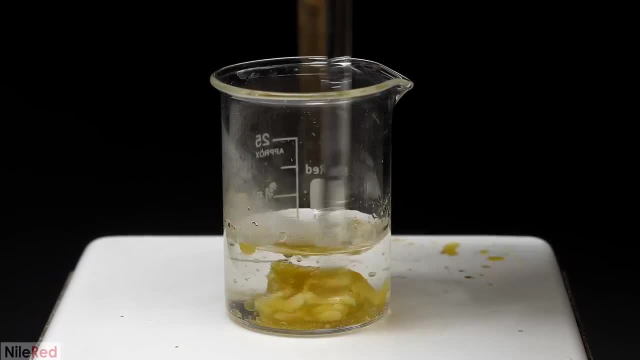 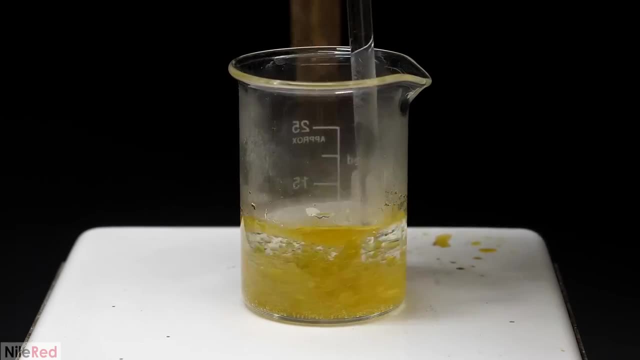 used a slightly different method For this one. I added about 10 mils of water and brought it to a boil. I'm not exactly sure at what temperature this happened at, but eventually the raspberry ketone melted into an oil. 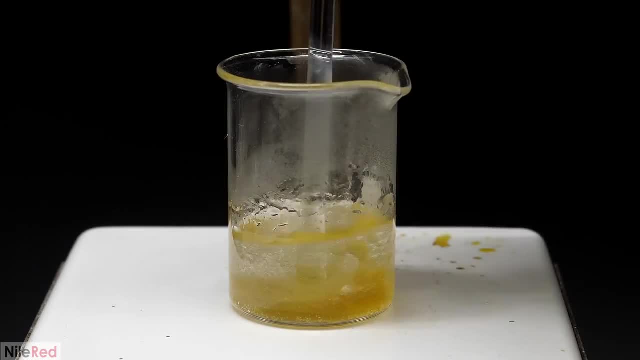 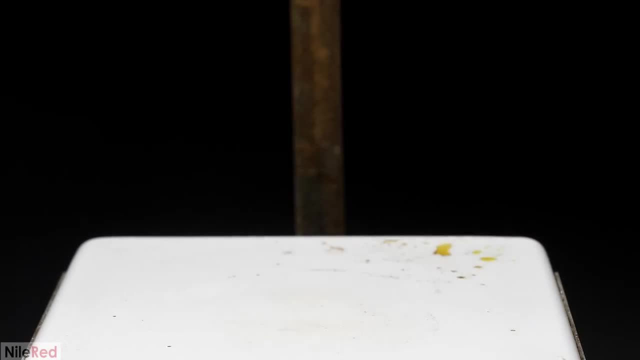 Pure raspberry ketone has a melting point around it. It's around 82 to 84 C, so this happened probably in that area. I then boiled the water for a couple minutes and I took it off the hot plate. I let it cool back to room temperature, but no crystallization happened and it just stayed. 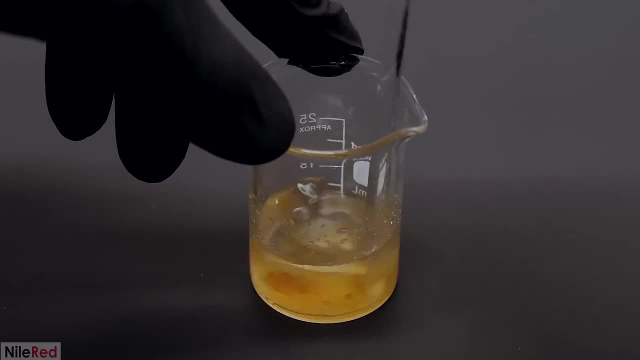 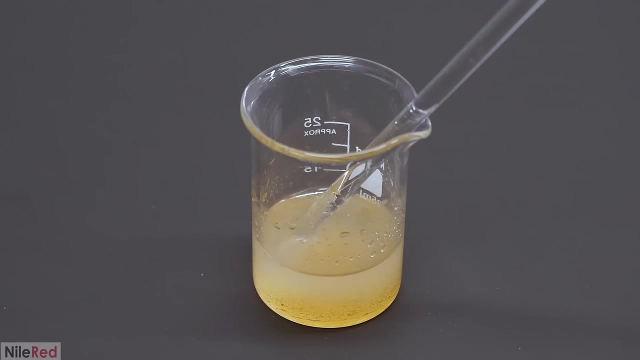 as an oil. Some chemicals can kind of be annoying, like this. I mean, we saw that it was a solid before, but now that it's at room temperature again, it decided to stay as an oil. I had to force it into being a solid again, and to do this I put it in the freezer. 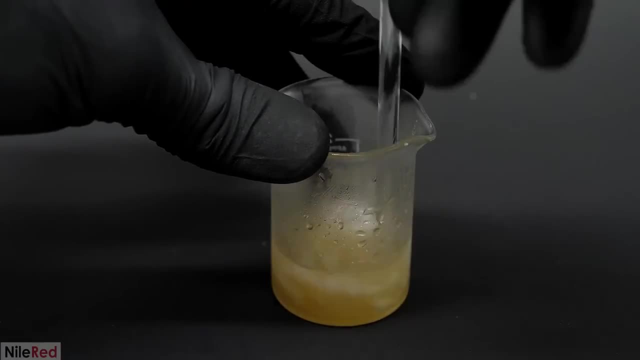 I waited till the water, and then I put it back in the freezer. I waited till the water just started to freeze, and then I took it out and mixed it around. At first it looked like it was still pretty stubborn and not much was happening. so I 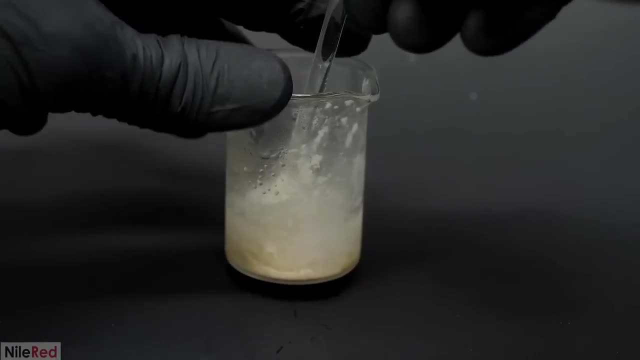 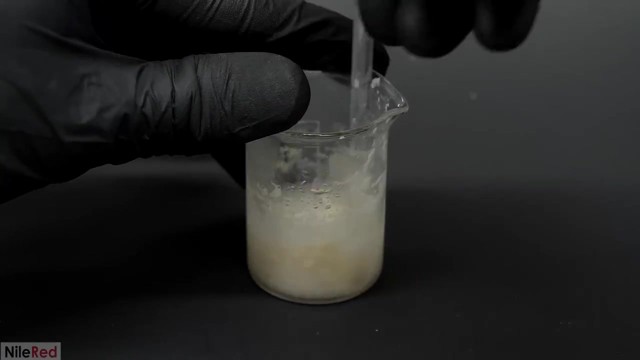 kind of gave up and turned off my camera, But then, of course, when I wasn't filming it, it decided to solidify Over the next couple minutes. I did my best to try to break up all the pieces. The thin rod wasn't working very well, though, and I ended up changing it for a stopper. 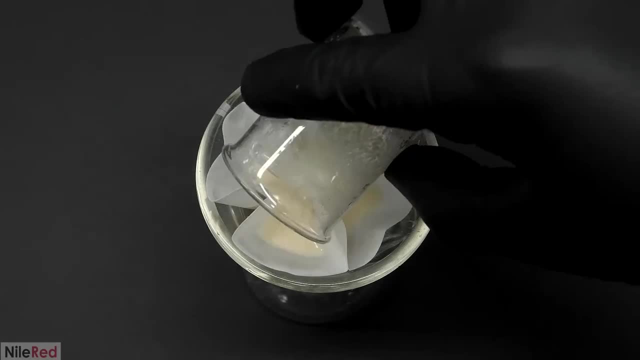 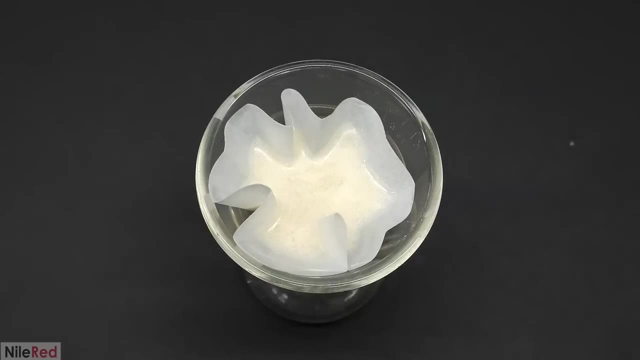 which was a lot better. All of the water was then removed by just a small gravity filtration. I also washed the beaker and the stuff in the filter with a small amount of extra water. When most of it was gone, I lightly squeezed it and I left it out to dry. This was what I had the next day and my total yield was 2 grams. This was extremely low, but I've done this procedure a couple times and I always get close to the same amount. I'm thinking that maybe my 4-hydroxymenzaldehyde wasn't very pure, but I'm not sure. I could also just be bad at chemistry, but I prefer not to do it. I'm thinking that maybe my 4-hydroxymenzaldehyde wasn't very pure, but I'm not sure. I could also just be bad at chemistry, but I prefer not to do it. 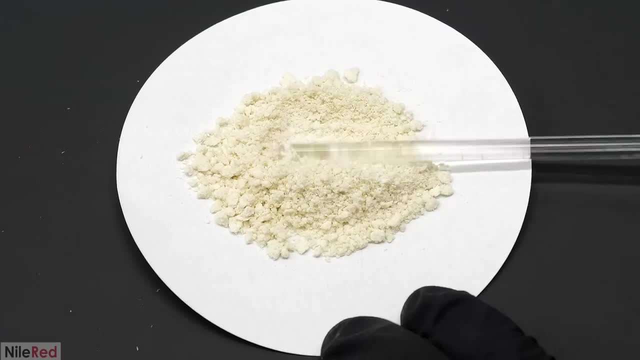 I'm thinking that maybe my 4-hydroxymenzaldehyde wasn't very pure, but I prefer not to do it. I could also just be bad at chemistry, but I prefer not to do it. The incredibly low yield aside, though, what did surprise me was how little this powder 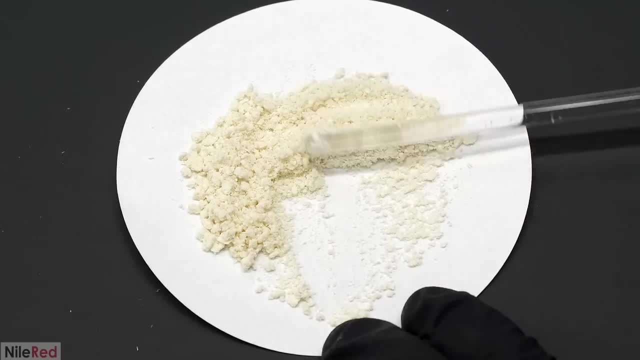 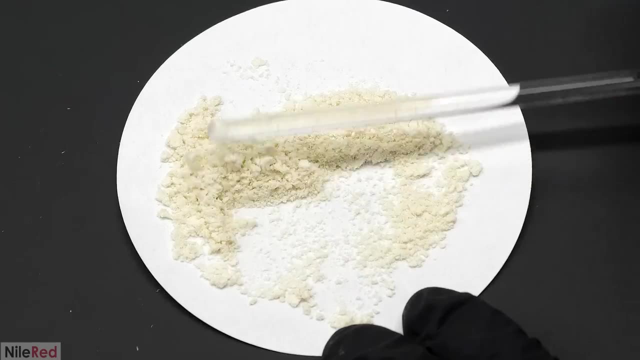 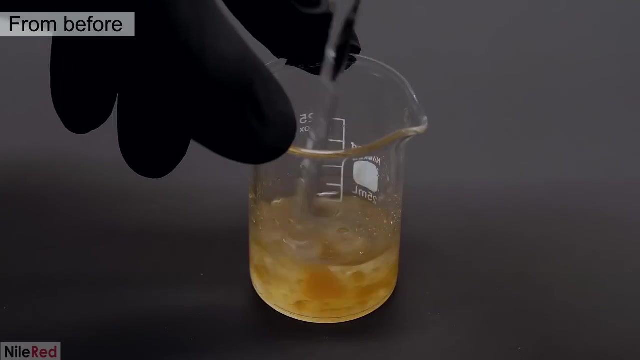 smelled. The odor was really faint and not overpowering at all, unlike some other compounds that I've made. I also wasn't getting any of that characteristic blue raspberry smell, and it was mostly just a sweet fruity one. Because I wasn't able to do a proper recrystallization, I wasn't sure how pure this stuff was. 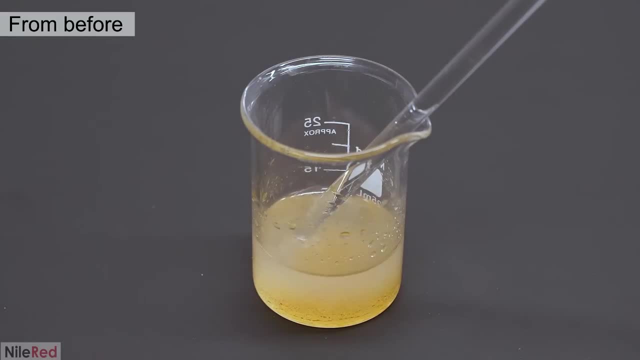 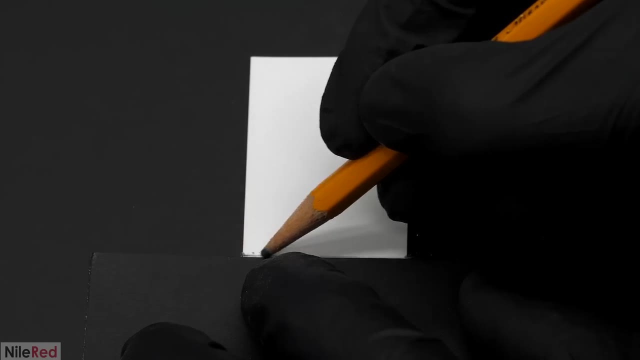 I was also a bit concerned because when something fails to crystallize, it can sometimes mean that there are a lot of impurities present. To figure out its rough purity, though, I just had to do something called TLC. To do this, I first needed a reference sample. 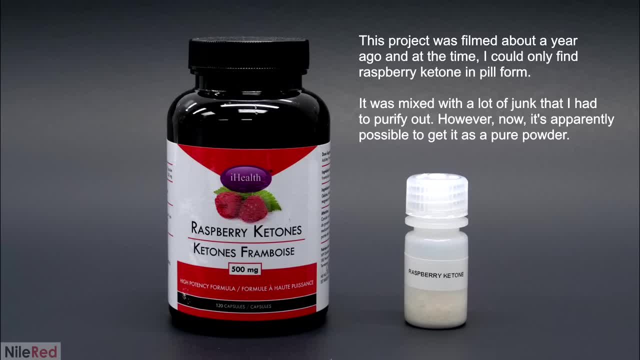 which, for a lot of projects, can be hard or impossible, but in this case it was really easy. As I mentioned in the intro, Pure Raspberry Ketone is sold online, so I just had to pick some up. Then, onto a TLC plate, I loaded a very small sample of this along with some of the stuff. 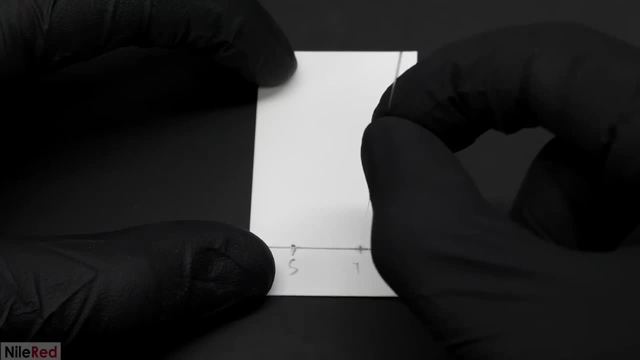 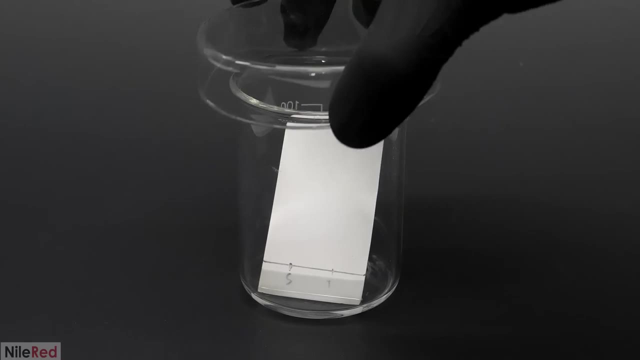 that I made. This was done by dissolving each of them in a small amount of acetone and they were applied using a very thin capillary, And when it was ready, I put it in a beaker that was preloaded with a 50-50 mixture of hexanes and ethyl acetate. I originally planned to do a small 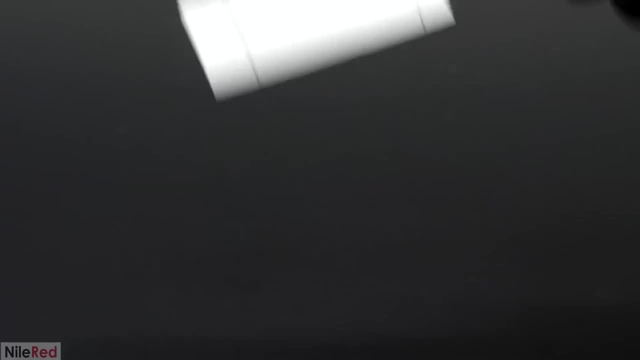 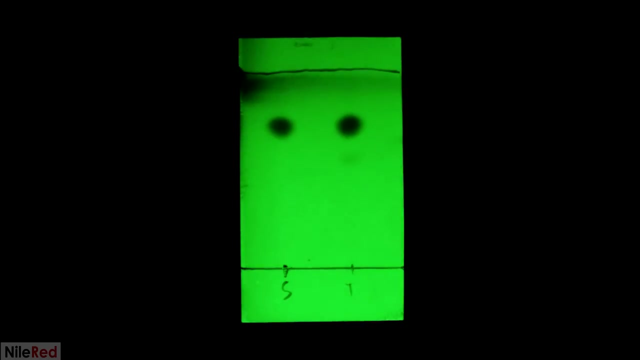 little TLC tutorial here, but this video has already turned out to be way too long, so I'm just going to show the results. When I looked at the finish plate under UV light, I saw that the spots were the same size for both. the reference: 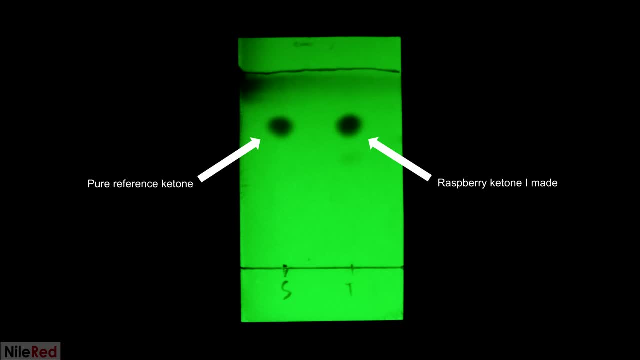 and the TLC plate. so I decided to go with the TLC plate. Then the test, and they travelled the same distance. This confirmed to me that, besides just going by smell, I did make Raspberry Ketone, Also because there was little to. 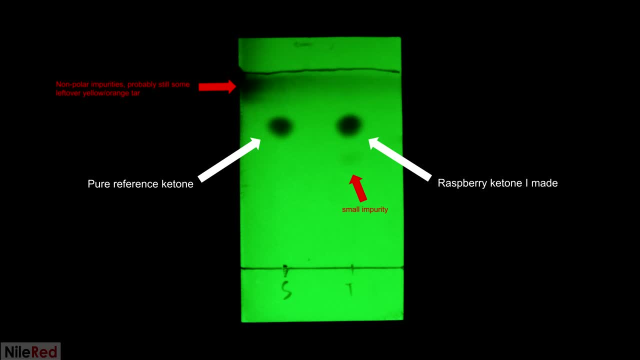 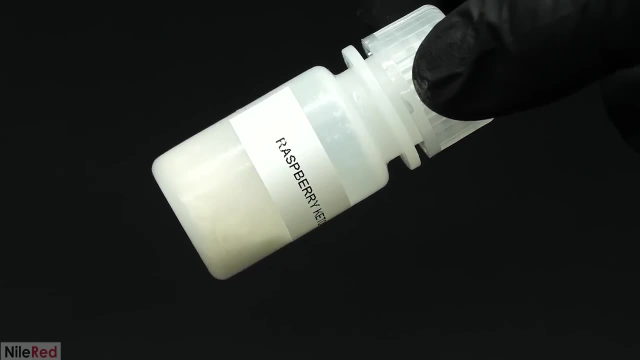 nothing else on the plate. it told me that it was relatively pure. Now, with all that confirmed, I felt comfortable moving on and trying to make the perfume. I initially thought that this might be a bit complicated, but I quickly found out that the 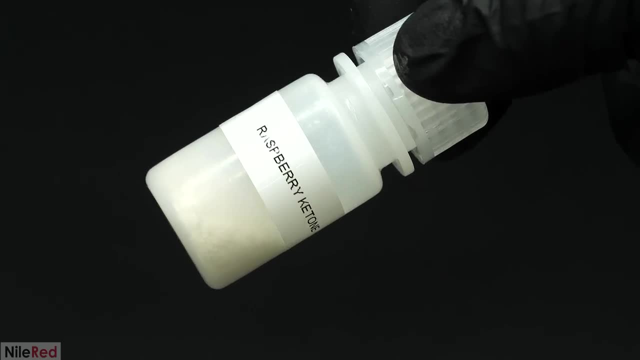 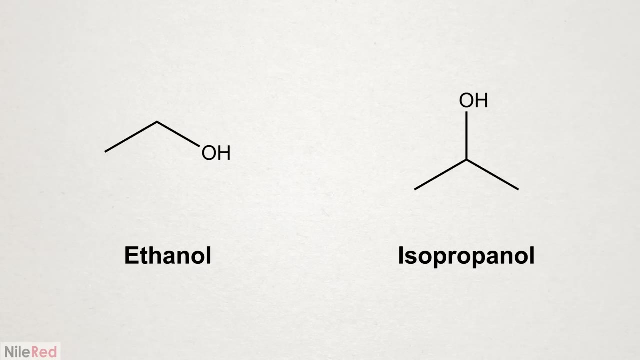 general idea of perfume is actually really simple. You basically just need to take all the aroma compounds that you want and mix it with a carrier solvent. There are many different carriers that can be used, but the most common ones are just simple alcohols like ethanol or isopropanol. 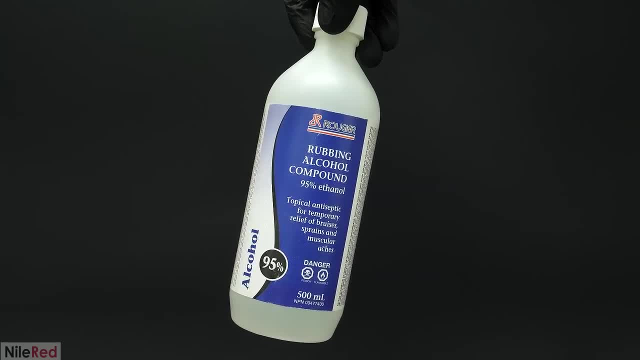 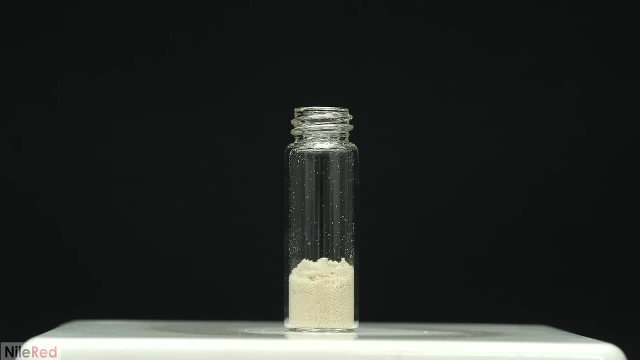 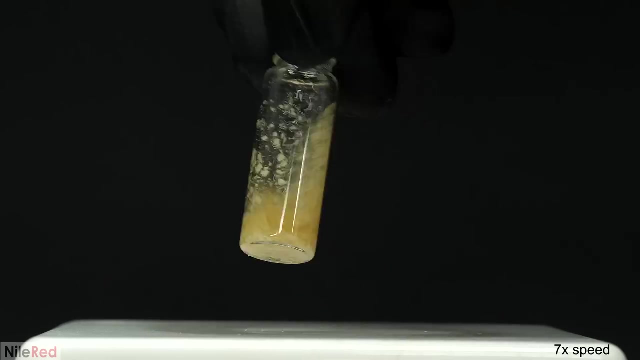 I went with 95% ethanol because it works well, but also because it's cheap and easy for me to get and it's sold at my local pharmacy. So, to get started, into a small vial I added about half a gram of the ketone. Then I added the ethanol in small portions. I wanted to go. 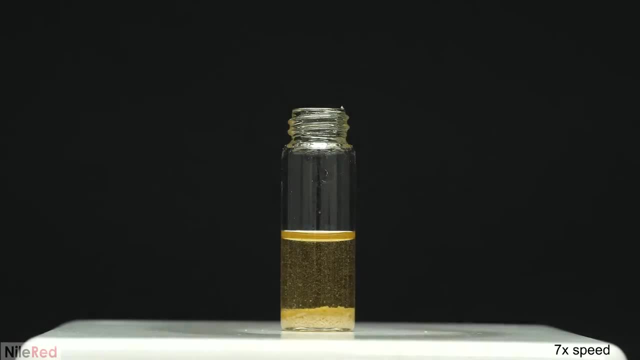 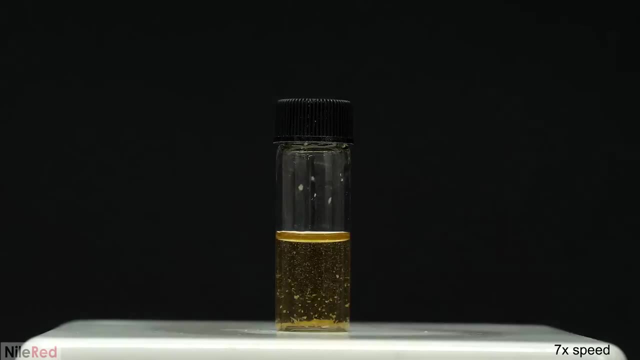 just until the point that it all completely dissolved. I did this because I had no idea how potent it was going to be as a perfume, so I wanted to make it as concentrated as possible so I could dilute it later, if I needed to, After a couple minutes, with more ethanol and a bit of 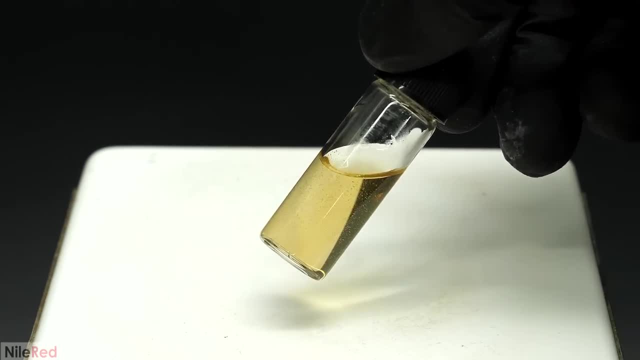 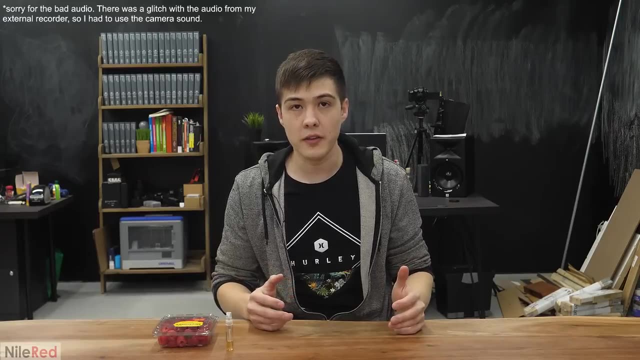 shaking. it all disappeared and I was well basically done To test it. I poured it into a small spray bottle and I shot the back of my hand After letting the ethanol evaporate for something like a couple minutes. I can try smelling it, but I don't think it's going to work, So I'm going to. 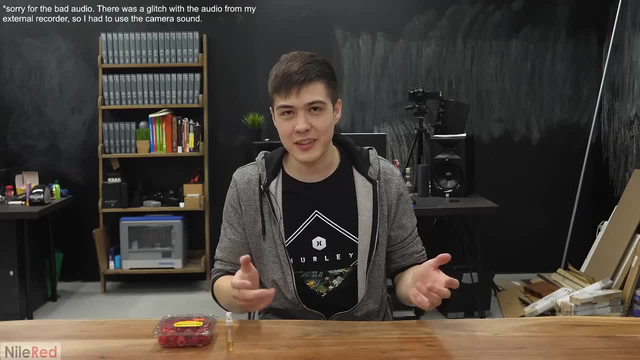 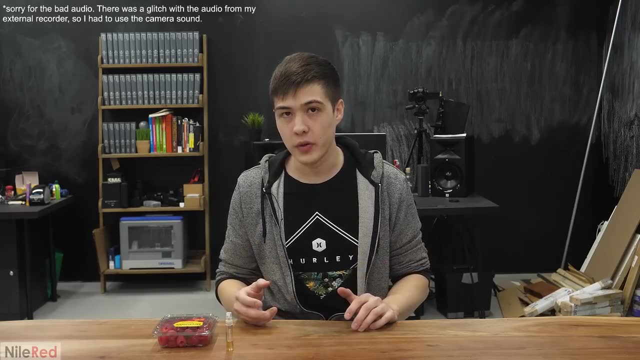 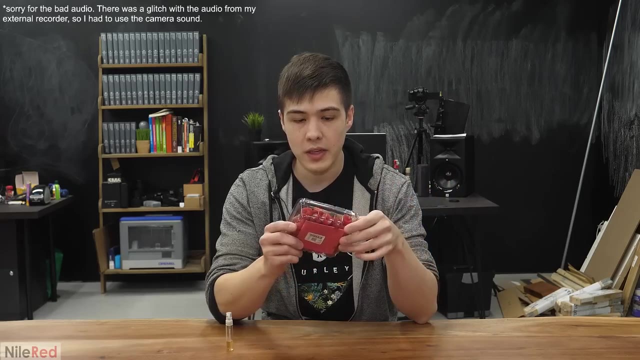 spray it and it smells exactly like the dry powder did, which, I mean, doesn't really surprise me. It's just faintly sweet and kind of fruity, but it doesn't smell like raspberries, And I kind of expected this, because, when it comes to artificial scents and flavors, if you just pull 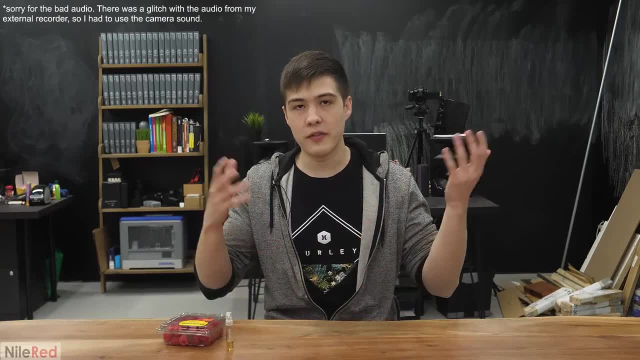 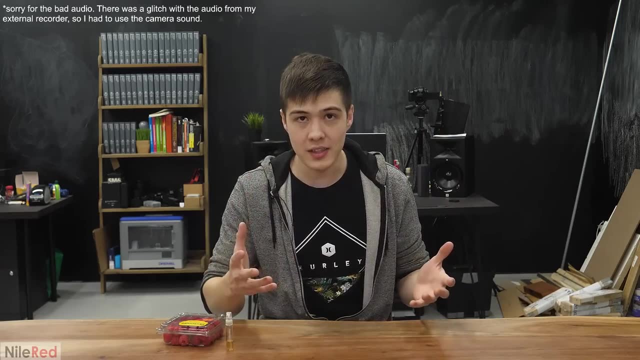 out the major component from the fruit, the vegetable or whatever you're trying to mimic, it's not going to be the same. You're going to get just one fraction of the complex smell or taste that you're trying to get. So for raspberries, 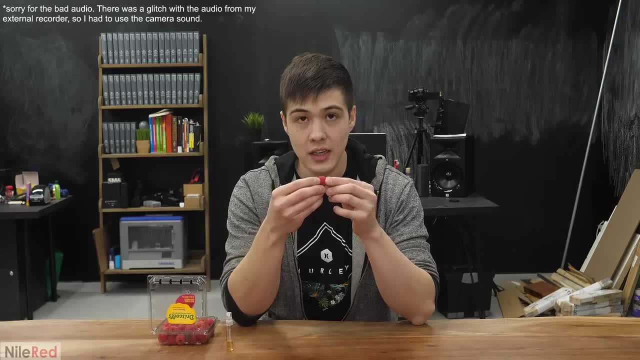 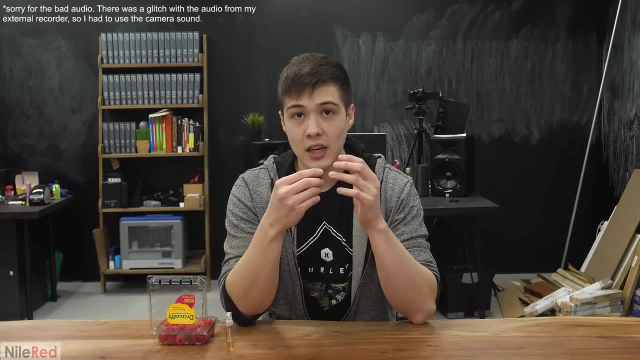 I can try smelling this here and it smells very different than the ketone, which is supposed to be its major component, but it's just missing a lot of other things which give the raspberry its characteristic smell. So when you're trying to make an artificial flavor, 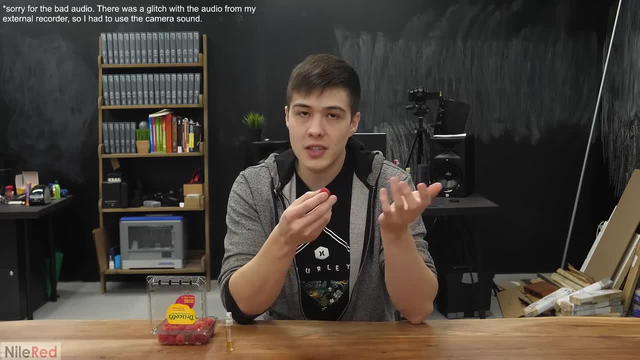 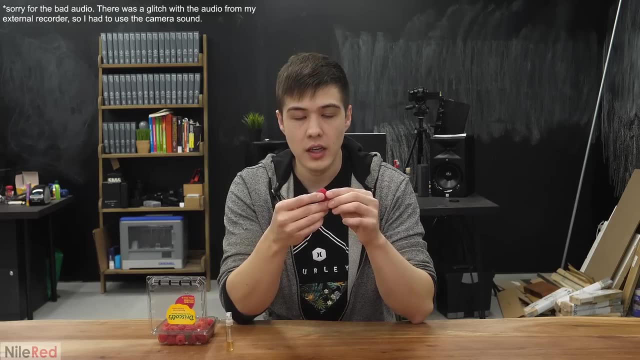 or smell. it can be quite difficult. You can sometimes get away with just using a couple, but you'll often need several or even a dozen chemicals to get close to what you're looking for. There are, however, some exceptions to this, like with vanilla, which can be mimicked. 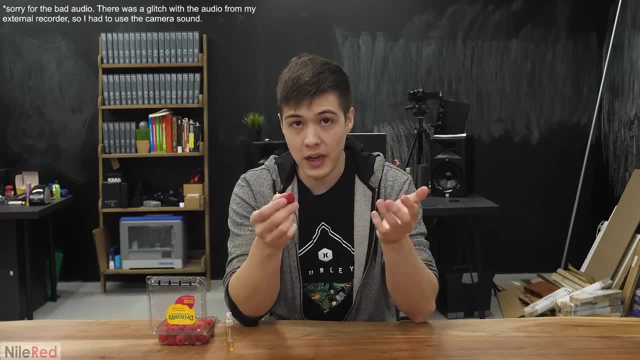 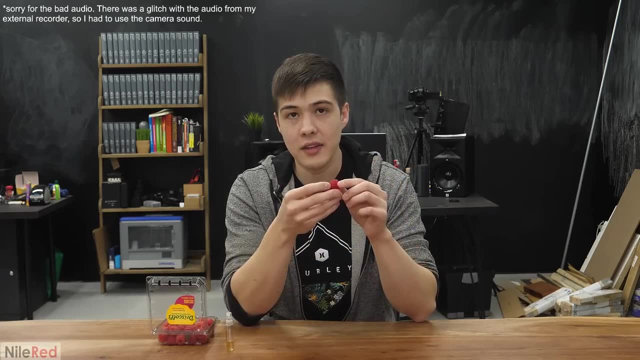 pretty well by just synthesizing its major component, which is vanillin, And that's what's used to make most artificial vanilla extracts, and most people can't tell the difference between that and the natural one. Anyway, I think that's about the end of this project. 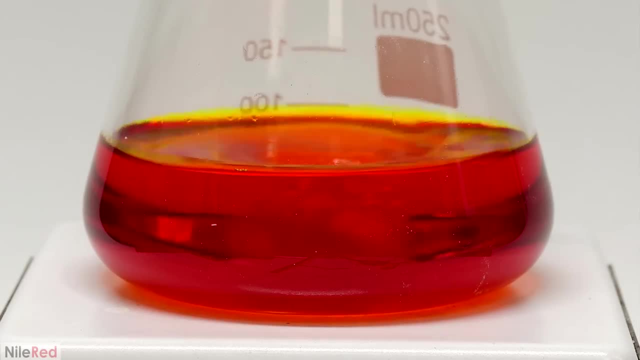 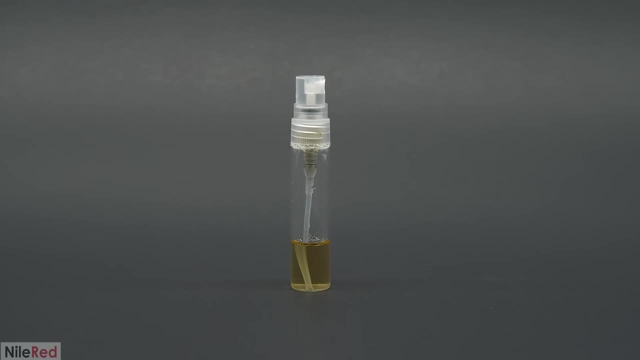 I honestly had a lot of fun with it, but making the raspberry ketone from scratch wasn't very efficient. I ended up really liking the perfume part, though, so I think in the future I'm gonna try to make some more smelly compounds. However, I think I might venture away from nice.